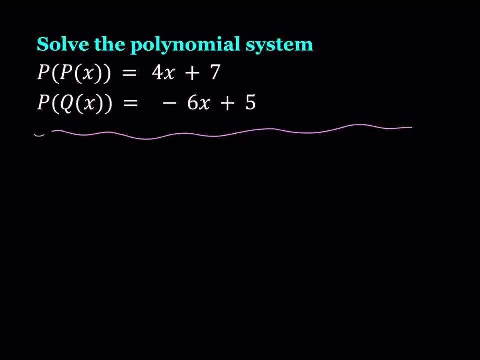 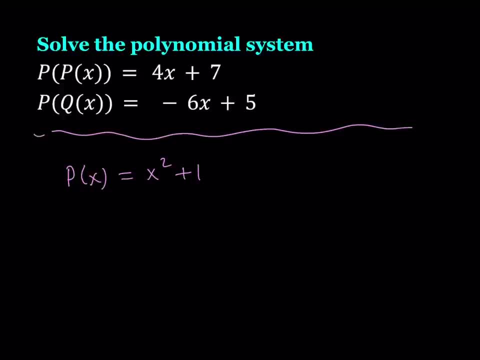 into, I don't know, t of x or something like that, or a of x. How about that? Let's do it so people don't get confused. They're going to say: how did you change the p of x? Okay, let's suppose we have. 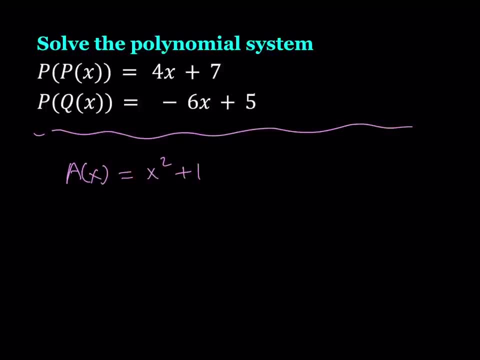 a polynomial. a of x equals x squared plus 1, and I want to compose a with itself, So it's kind of like a of a of x. How do you evaluate that? Well, just replace the x squared plus 1.. So I'm going to. 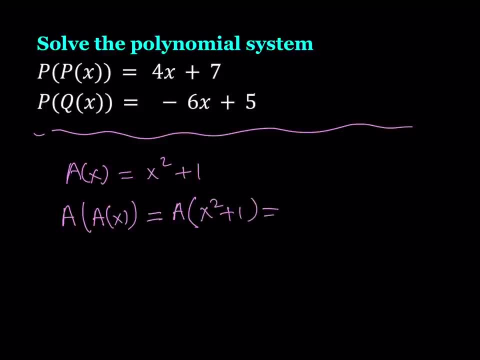 do x with a of x, which is x squared plus 1, and by using the definition of a of x. this gives you x squared plus 1, squared plus 1.. And then, from here, you get x to the fourth power, plus 2x squared. 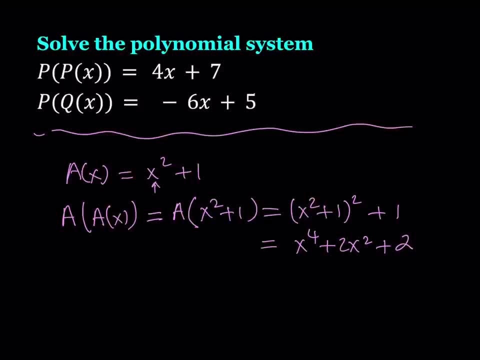 plus 1 plus 1 is going to give you 2.. So now notice that when I compose a with itself, I got a quartic polynomial. a was quadratic, then the degree just doubled. If I take a cubic and compose it with itself, I get a quartic polynomial. So I get a quartic polynomial, So I get a quartic polynomial. 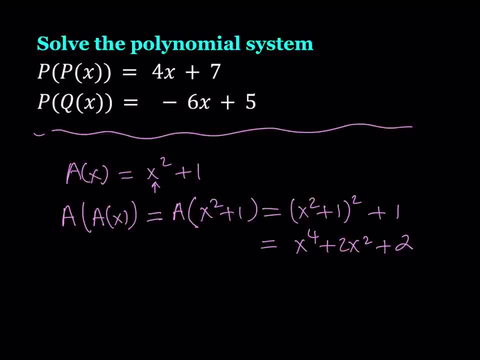 with itself. I'm going to be getting something 6 power, So it's basically going to well, I shouldn't say double. So if you had a cubic polynomial, let's. let's think about another scenario, like: suppose b of x is equal to x cubed, then b of b of x would be b of x cubed, and that would equal. 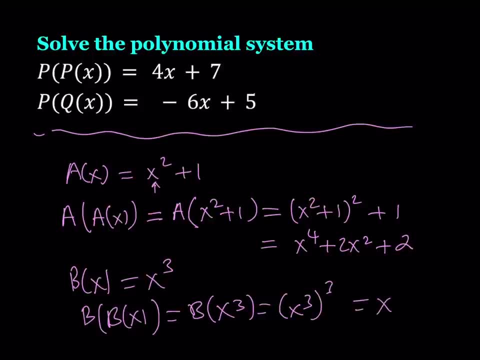 x cubed, quantity cubed, and that will be x to the ninth power. So the power basically is the square of the degree. So now, here we have a linear result. What is that supposed to mean? The degree of this polynomial is 1 and the square root of 1 is 1.. That means that p of x needs to be. 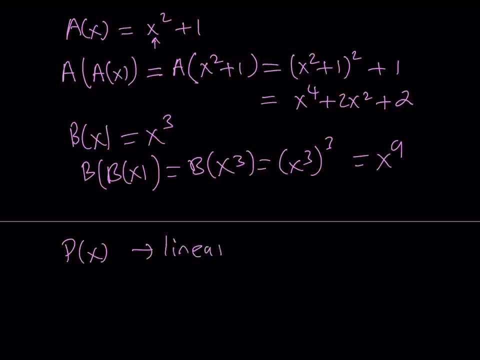 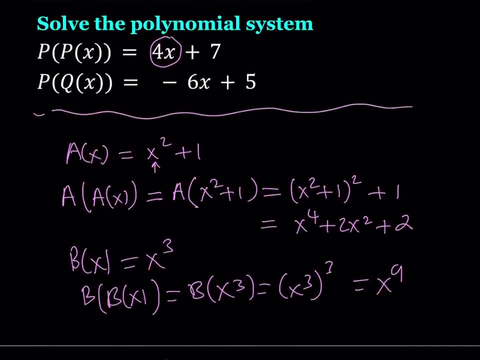 linear. All right, so that's the first assumption we have to make. Otherwise we're going to have to go through infinitely many possibilities and obviously none of them is going to work except for the linear case. So p of x needs to be linear. Let's go ahead and solve the first equation first. 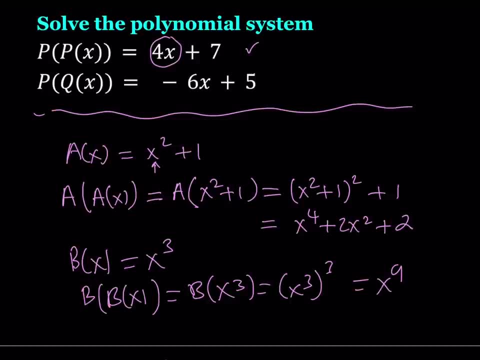 This is not something you can do elimination or substitution with. yet Let's go ahead and find out p of x first. So if p of x is linear, can I write a square root of x cubed and a square root of x cubed? 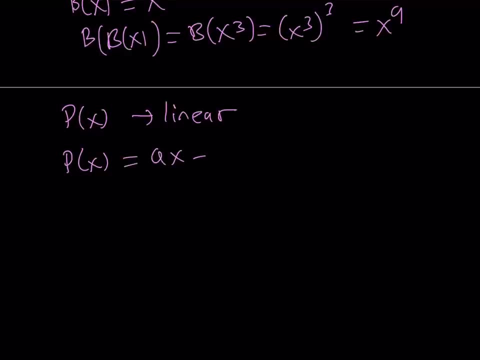 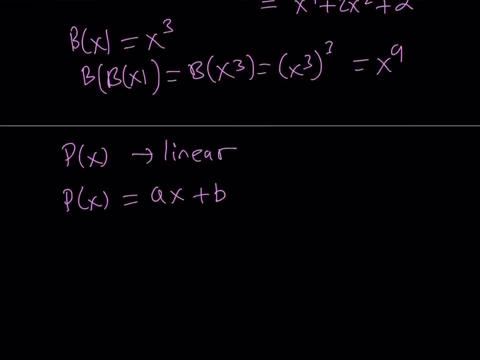 Let's write it as ax plus b, right, where obviously a is not equal to zero, so on and so forth. Now, if you compose p with itself, which is p of p of x, we're supposed to get 4x plus 7.. Now replace p. 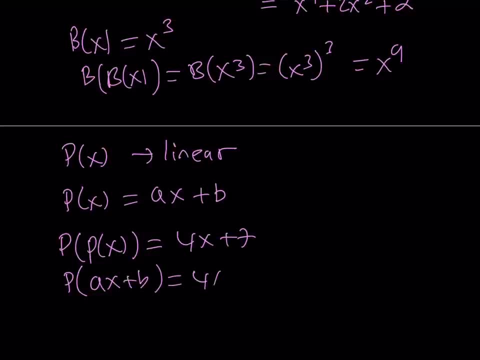 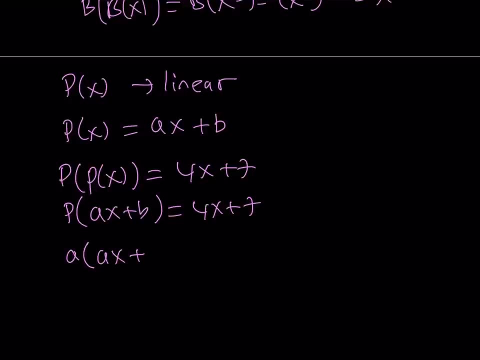 with ax plus b and you're supposed to get 4x plus 7.. Now apply the definition of p to ax plus b. so that's going to be a times the quantity ax plus b plus b. So that's going to be a times the quantity ax plus b. So that's going to be a times the quantity. 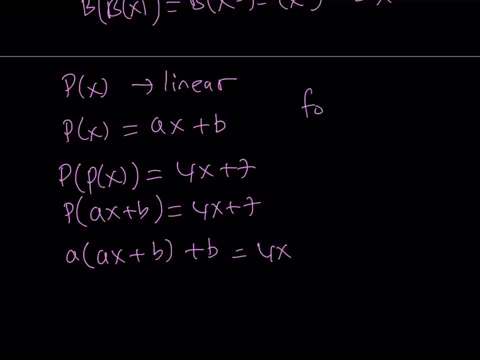 and you can keep doing this. Sometimes you're going to have a problem like f of f of f of dot, dot, dot n times. That's basically what it means, Okay, and of course, in these cases, hopefully there's some type of pattern, otherwise it's going to take, it's going to be crazy. All right, so let's go ahead and 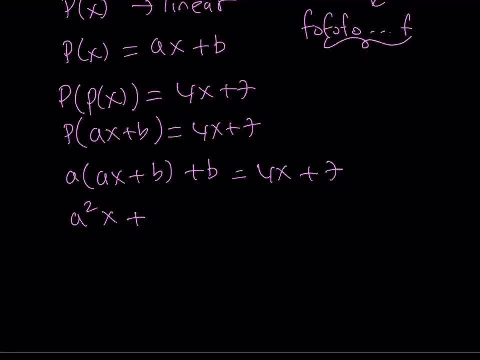 distribute a squared x, and then I get a b plus b. Let's go ahead and factor out b, so it's going to give us a plus one. in parentheses. This is going to make a solution easier. So now we have the following: And what is that supposed to mean If two polynomials are equal for all values of x? 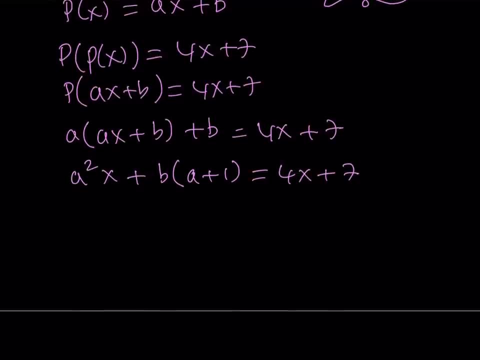 that means the coefficients of x are equal and the constant terms are equal. So from here we get two results: a squared equals four. That means a is equal to two or a is equal to negative two. Obviously there's no reason why we would pick one over the other, So we're going to consider both If a is. 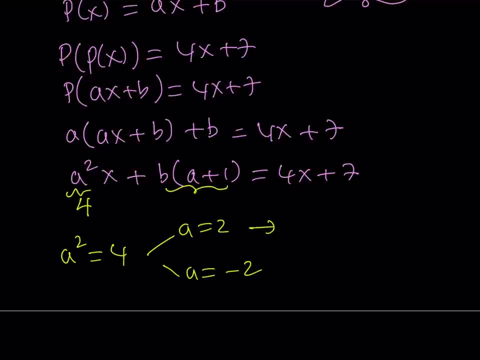 equal to two. I can just go ahead and substitute that here. Well, this is supposed to equal seven, and if a is two, then I'm getting something like three. b equals seven, and this implies that b is equal to seven thirds From the second one. I get a nicer. 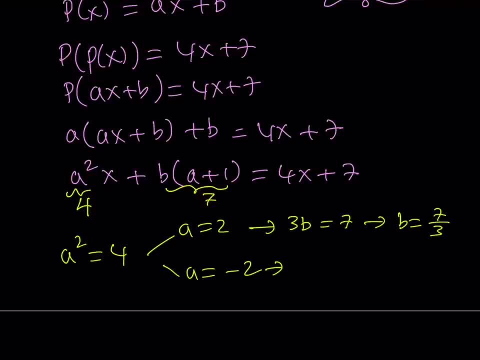 expression: If a is equal to negative, two negative two plus one is negative one. So I get negative b equals seven, which implies b equals negative seven. So this a value should be taken with that b value and the second one should be taken with the second value. So this gives us two options. 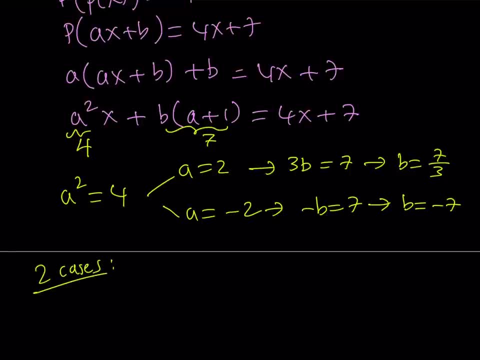 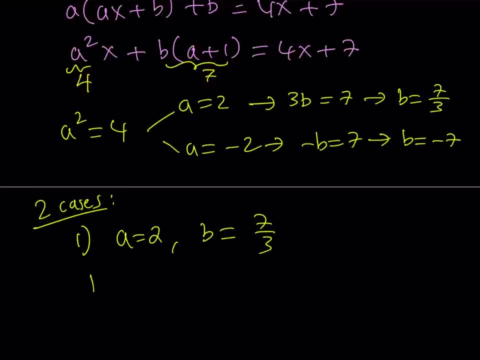 Okay, two cases. Let's take a look at both cases. Case number one: Case number one is where a is two and b is seven thirds, And that gives us p of x equals two x plus seven thirds. Now you can obviously test this like plug it in, For example, if I had to do the composition of this with itself. 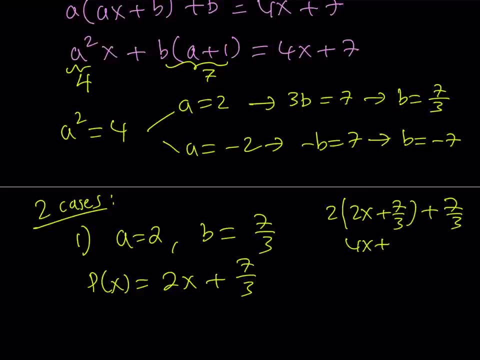 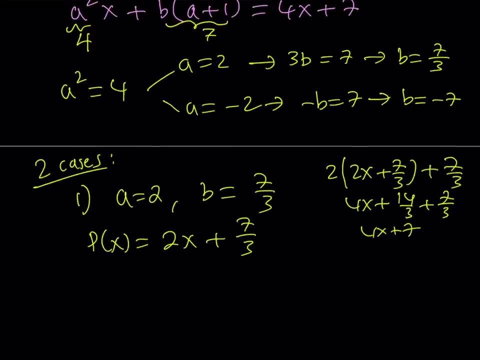 you'll notice that it works. You get four x plus 14 thirds plus seven thirds, which is 21 thirds, and that is equal to seven. And obviously the other one is going to work as well, So you can test it. You don't have to, but it just shows you that you got it right. 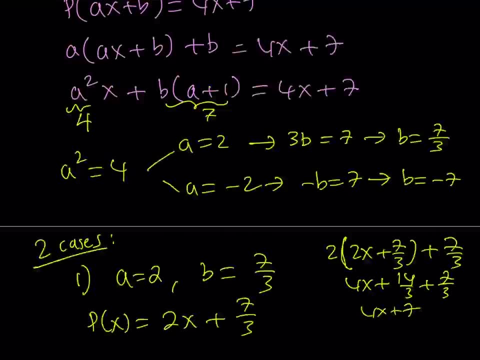 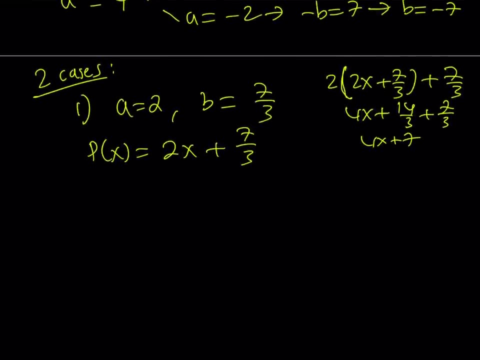 Now, p of x can be this one. and what about the q of x, right? Well, p is composed with q, and you know the composition is from right to left. So p of q of x. Let's go ahead and write that down as an. 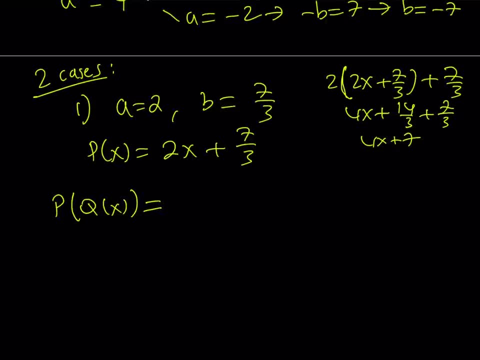 equation P of q of x is given to us as negative: six x plus five, right? So we're supposed to find q of x from here, where, when p of x is equal to two x plus seven thirds? So let's go ahead and apply the definition of p to q of x. That gives us two times two x plus seven thirds. So let's go. 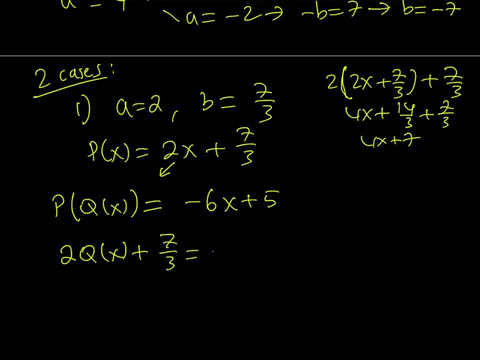 ahead and write that down. So p of x times q of x plus seven thirds is equal to negative six x plus five. Obviously there's more than one way to do it. You could also assume that, hey, q of x must be a linear polynomial as well, And suppose we call it mx plus n Substitute. solve for m and n, and so on. 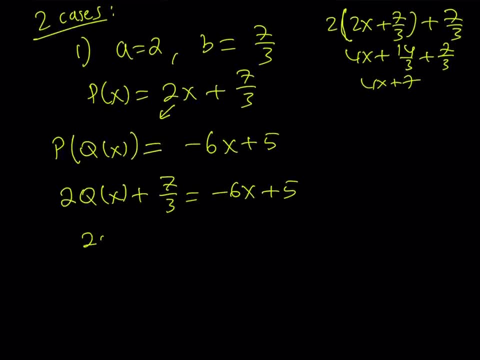 and so on, But I just wanted to do it this way because it's kind of cooler. Anyways, so you can go ahead and solve for q of x: Isolate it Subtract seven thirds. Fifteen minus seven is eight, So it's going to be negative six x plus eight thirds, And then you can just divide it by two, So you 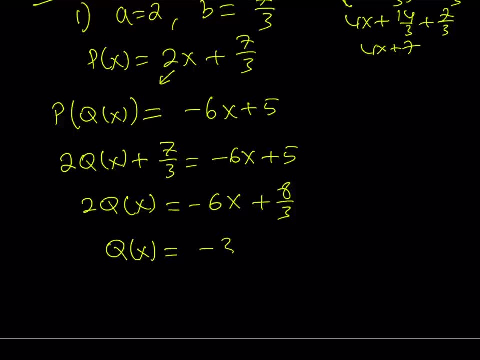 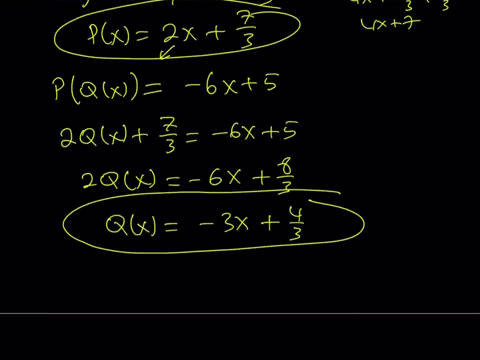 divide everything by two here to find q of x, And that is going to be negative three x plus four thirds. So for this p of x value we get this q of x value. That gives us a solution as an ordered pair And we're going to write these at the end, So don't worry about keeping track of them, right. 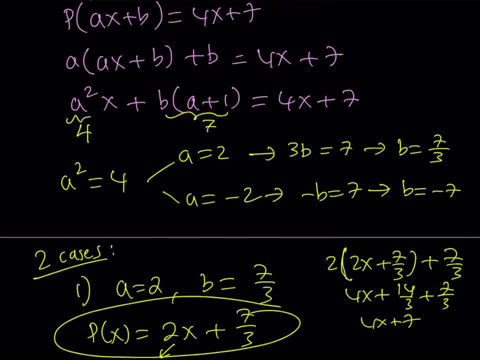 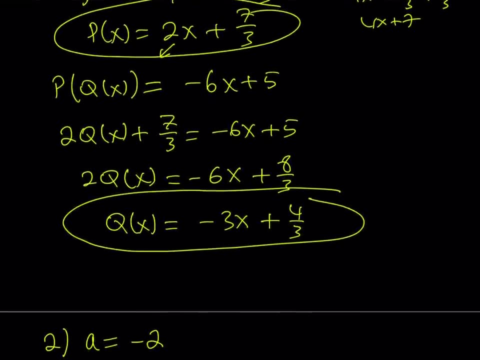 now Let's go ahead and take a look at the second case. Now, remember, the second case involves a being equal to negative two. So if a is equal to negative two, then this gives us what It should give us: a solution. It was: b equals negative seven- Great. So b equals negative seven in this case, So that